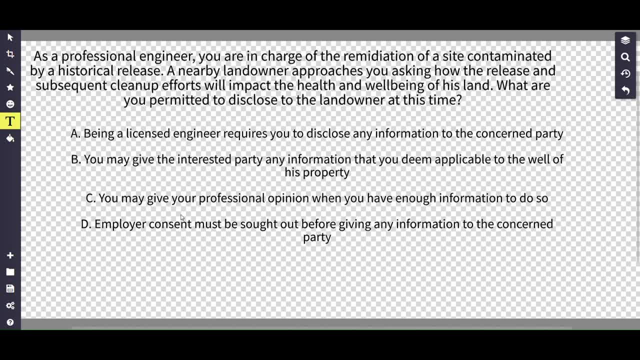 engineering. that you'll kind of learn is it's an easy concept. that doesn't necessarily mean that it's simple. A lot of ethic questions really rely on choosing the best answer, and sometimes the questions can have a good answer, but there is a better answer that could. that is the actual answer. 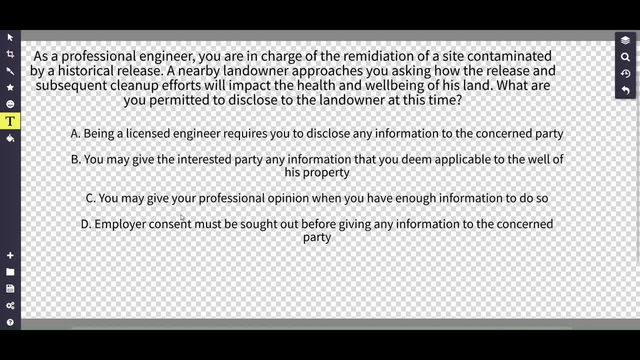 So you'll see what I'm talking about as we dive into more and more problems. Just make sure that you're pausing the video, trying to do it on your own and then trying to follow along afterwards to see, maybe, where you went wrong or maybe you have a dispute and you can leave it down in the comments. 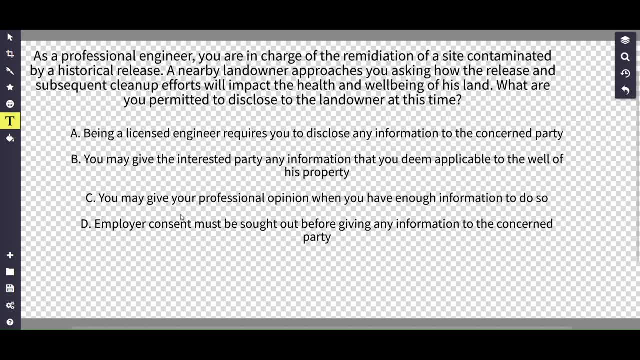 So go ahead and pause right now, but for the rest of us we're going to jump right in. So the question here is asking: as a professional engineer, you are in charge of the remediation of site contaminated by historical release. A nearby landowner approaches you asking how the release. 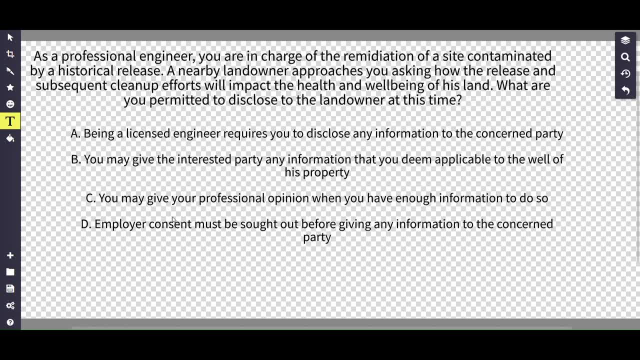 and subsequent cleanup efforts will impact the health and well-being of his land. What are you permitted to disclose the land owner at this time? So kind of answers that we have towards this particular question are down below, but just kind of dissecting what's being asked here. 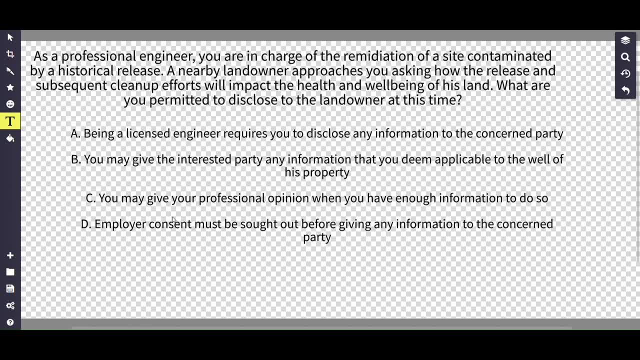 This kind of problem happens a lot when you're out and about. Mostly, you have to be an advocate for your employer, You have to be an advocate for the people, You have to be an advocate for the client that your employer is employed or being employed by, And so it's just one of these well balancing acts that you have to kind of figure it out, And thankfully there are a lot of step by step things you can do to kind of figure out those problems. 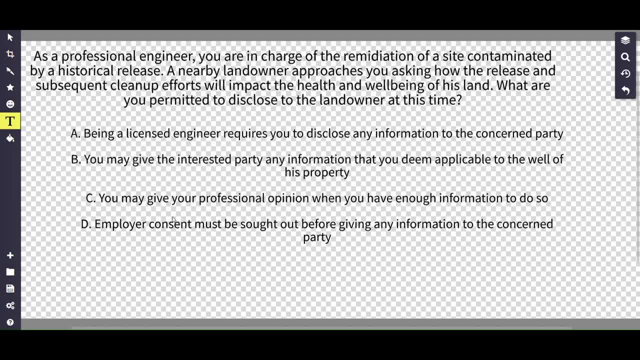 And if you were ever to be in this situation, just make sure to pause and just figure out the answer with your mentor, either going online, so on and so forth. These are all hypothetical in nature, So by no means should you actively try to put these questions in real life applications. They're more of a guideline, if you will. 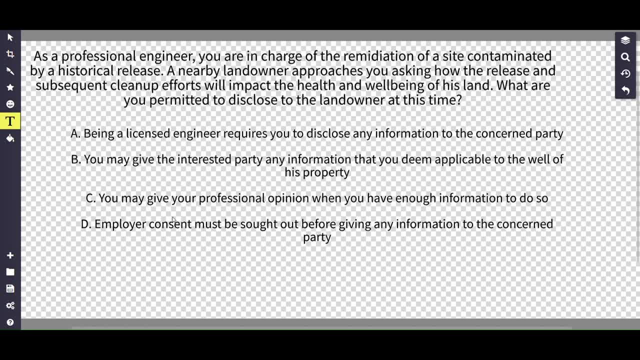 So for number A, we have being a licensed engineer required. So when we're looking at this, a big thing that we have to consider are: what are the laws that we are enforcing? So, like, what state are we in? What county are we in? So, other than state law, court, police, et cetera, licensees shall not reveal facts, data or other information obtained in a professional capacity without the prior consent of their clients or employer. 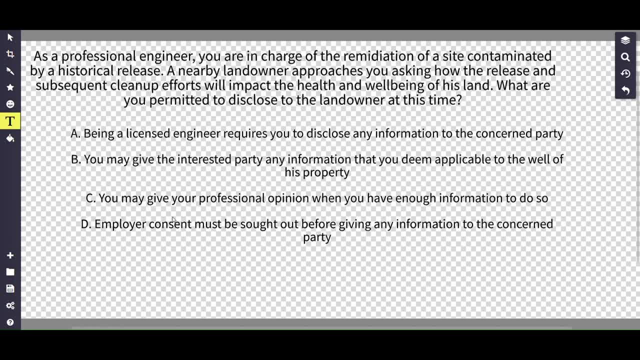 So it's just kind of one of those things where we have to protect the integrity of what we are trying to do. That's not to say that if there was an endangerment to the property, that you shouldn't go to the property. That's not to say that if there was an endangerment to the property that you shouldn't go to the property. 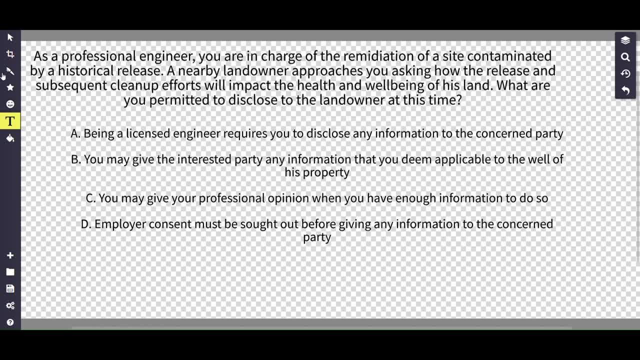 But in general we typically follow the answer of D as in dog, And so this right here is a good answer to kind of follow. Again, there are a thousand things that could go wrong in any situation, And so you'll have to analyze it And thankfully you can take a step back and say I really can't answer this right now, sir. 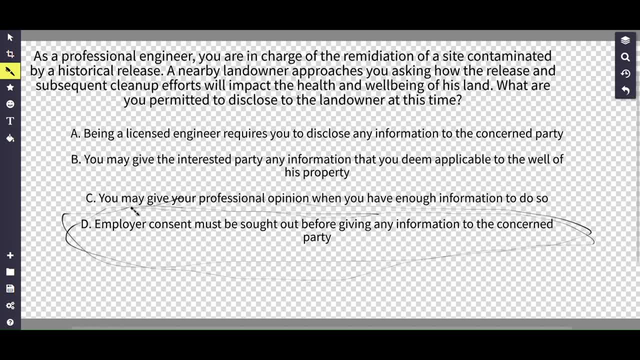 Let me get back to you. And then you can talk to your employer, You can talk with your mentors, You can even reach out to your old college teachers and see what's right. You can even look up your laws in that county, state or country that you're in. 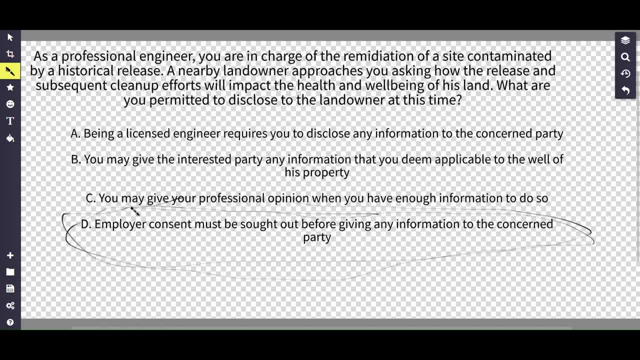 And it's just, ethics has such a wide variety, And so you might think that C is a good option where you give your professional opinion based, you know, when you have enough information. But again, D is the best answer when it comes to protecting the client, because that's what you were asked to do when you have to ask that permission. 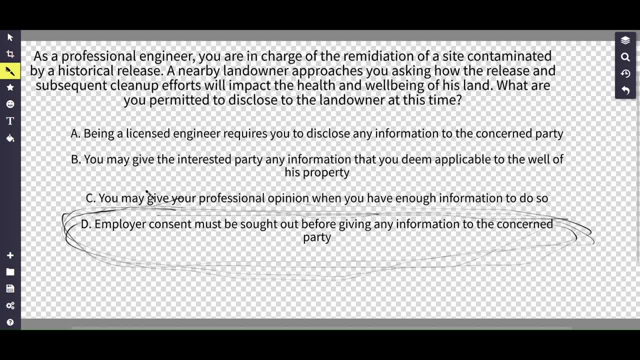 It's that integrity we're trying to uphold, so forth, And A and B D still is just the best option, And that really just kind of answers this particular question. So make sure you stick around and watch the next video. Hopefully you guys pause that. you guys had that video and you pause that video and you were able to get the right answer.